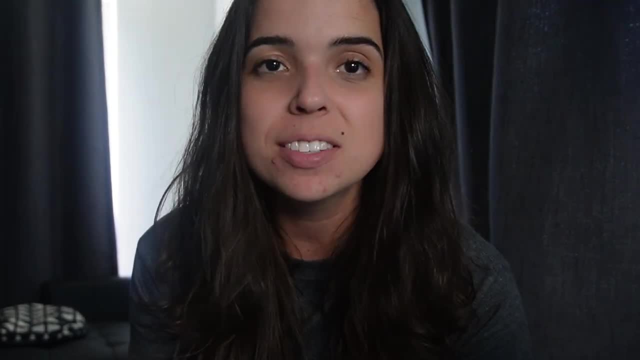 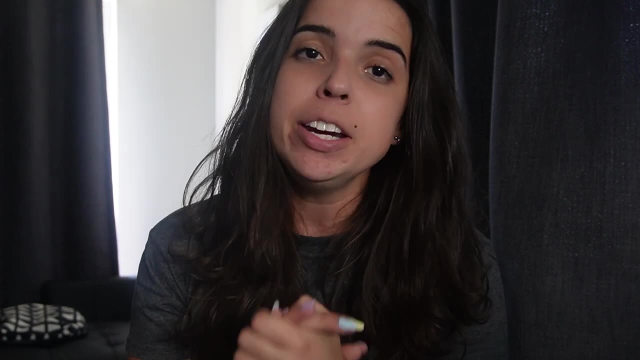 Hello, great tens, and welcome back to another video with me, Miss Martens. In today's video we're going to be looking at longitudinal waves and introduction. If you've missed any of my videos on waves, check out the description box below where I will link my playlist. Now let's jump. 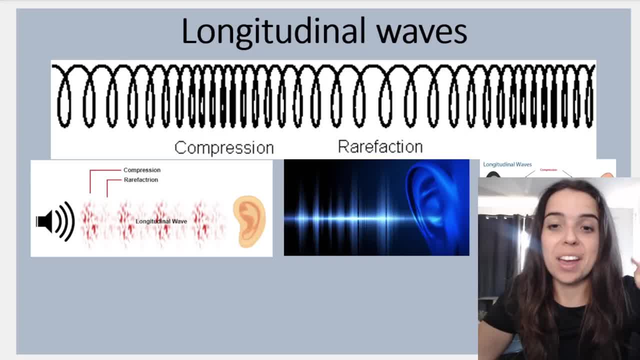 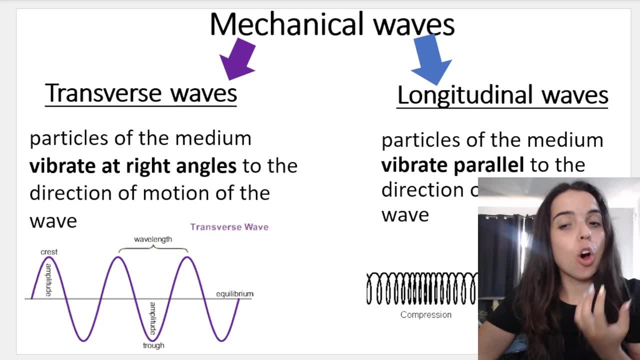 right into longitudinal waves. You can see a longitudinal wave behind me. Now, the first thing that you need to know- and I hope you've watched my other videos- is that longitudinal waves are a mechanical wave or they're a type of a mechanical wave. Now remember, mechanical waves are waves that. 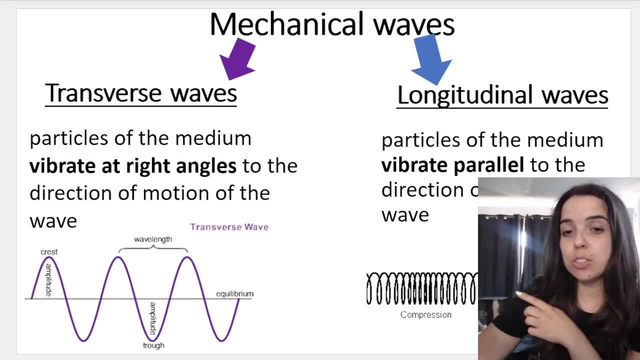 require a medium to travel through. We've got transverse waves, which I've already been through with you, and we've got longitudinal waves, which are behind me Now. sound waves are an example of longitudinal waves. Now, what makes longitudinal waves different to transverse waves? Remember: 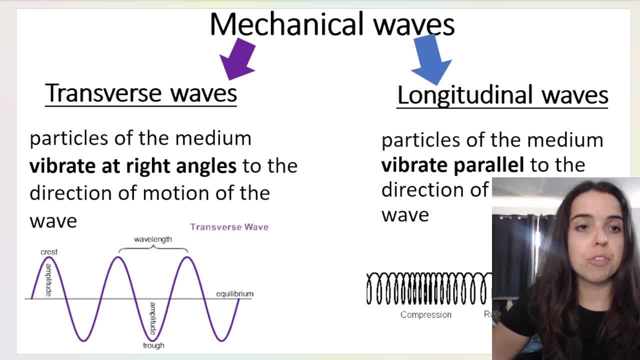 a transverse wave is a wave in which the particles of the medium vibrate at right angles, so 90 degrees To the direction of motion of the wave. So what that means, for example, is the particles of the medium or the particles of the air or the water, whatever, go up or down and the wave itself travels. 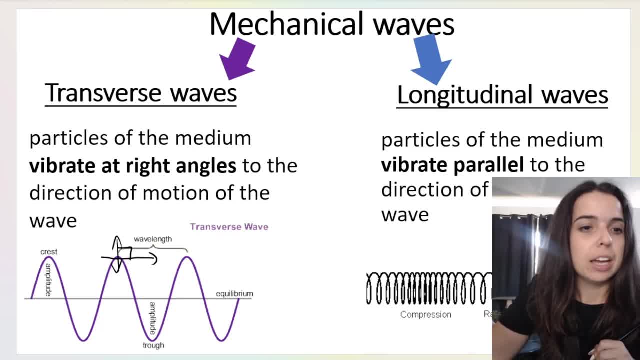 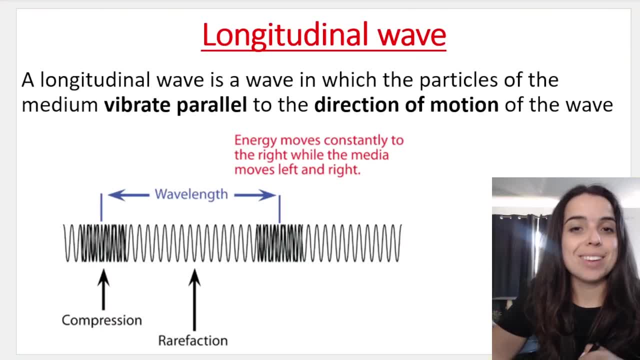 left or right. I hope you can see it's a 90 degree angle. And a longitudinal wave is different, because in a longitudinal wave, a longitudinal wave is a wave in which the particles of the medium vibrate parallel to the direction of motion of a wave. So a transverse wave is a wave in which 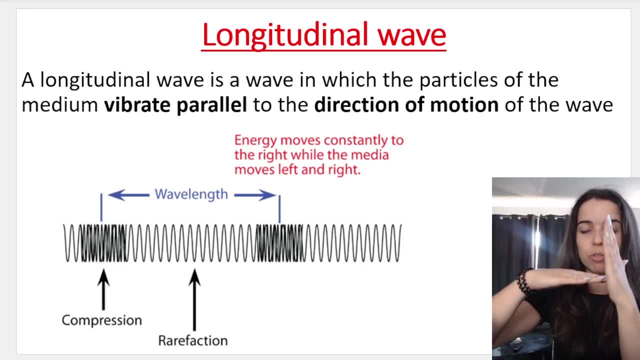 waves basically perpendicular, like those two. particles go up and down, if goes left or right along a two, nowhere is. particles move like this along the x axis, for example, and the wave travels like this along the x axis, so parallel to the direction of motion of the wave. So as you can see behind me, 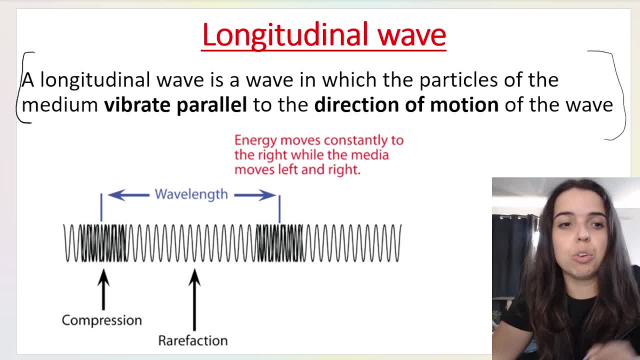 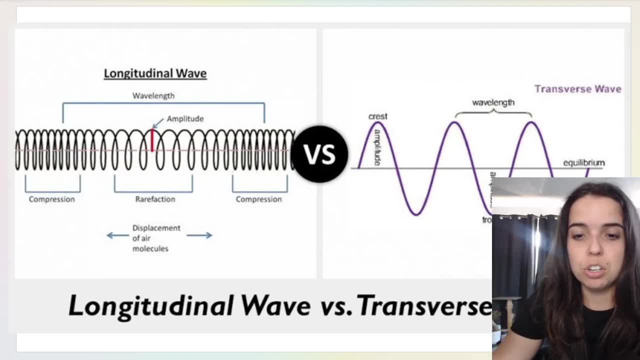 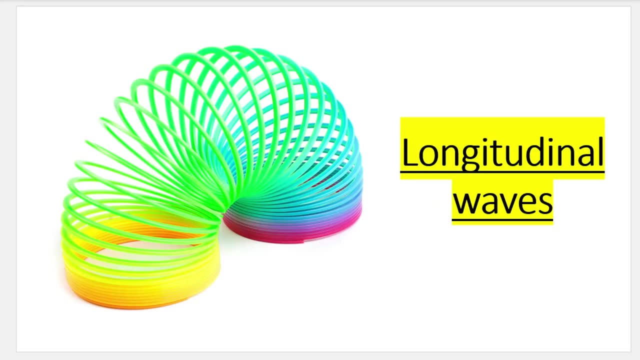 this. That's the definition for a longitudinal wave and this is what a longitudinal wave looks like. So here is another comparison between a longitudinal wave, a transverse way. Heroes where have just another diagram, illustrate some of the differences, And I want you to think of a longitudinal wave and the way. 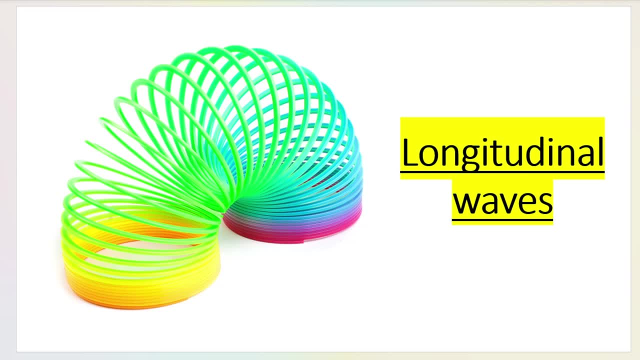 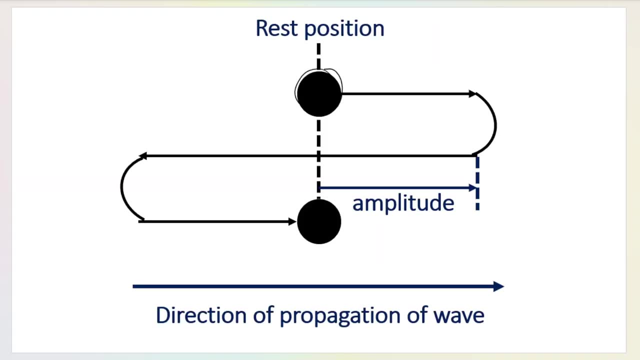 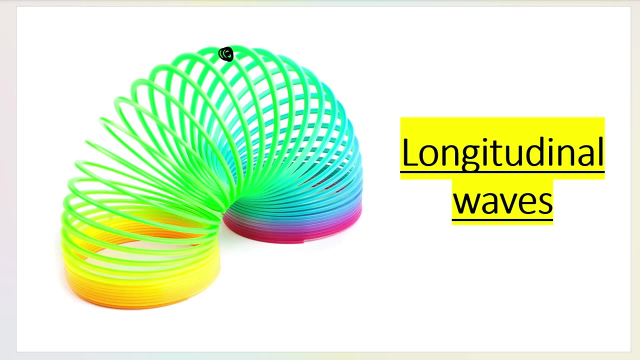 in which it moves as a slinky, almost. So basically, what ends up happening is the particles move like this. So this is a particle. this round dot represents a particle. This is the rest position of the particle. So think about a slinky. If I have to tie a little rope to the slinky, think 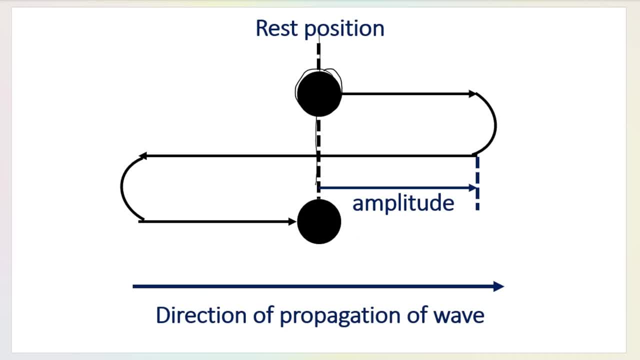 about it like this: The rope in the slinky. if I wiggle the slinky like that, move it back and forth. The rope will move like this: it'll bounce like that it'll move back to its rest position. it'll bounce in the opposite direction: move back to its rest position This distance over here. 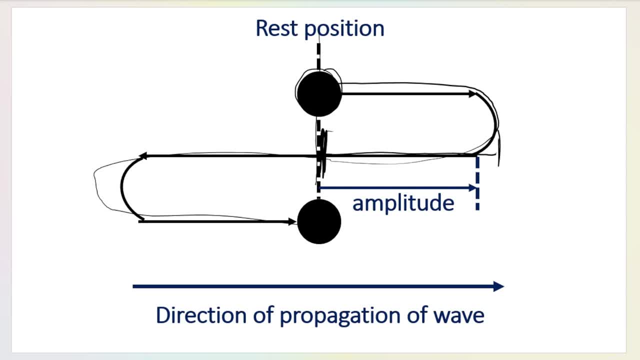 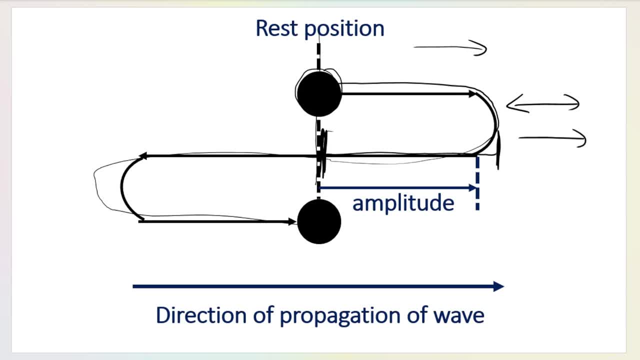 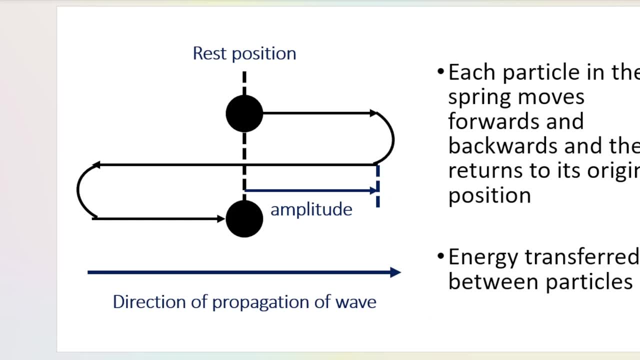 and right. the direction of the wave is left or right, So you can see that they are parallel to one another. So this is just an example. This is just showing you. each particle in the spring, or the slinky, moves forwards and backwards and then returns to its. 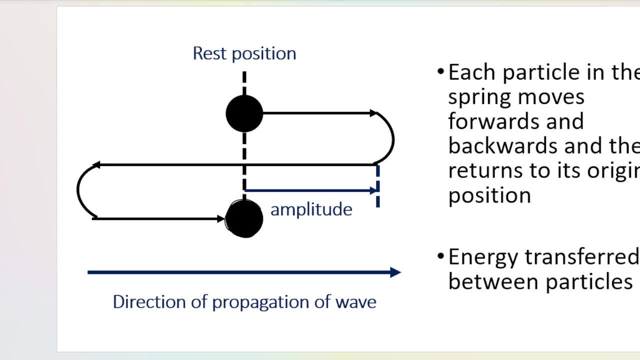 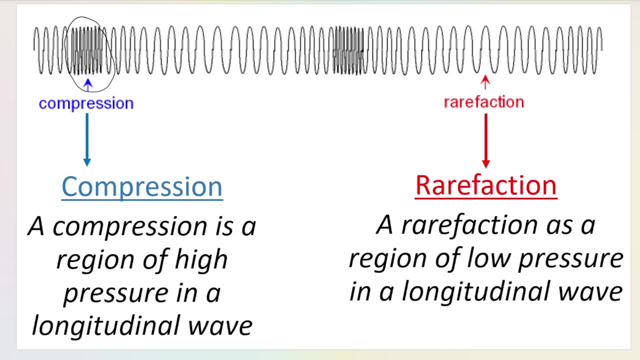 original rest position And when this happens, energy is transferred from one particle to the next. So remember, all waves transfer energy And what ends up happening in my wave is that I have areas of compression. So compression is a region of high pressure in a longitudinal wave. 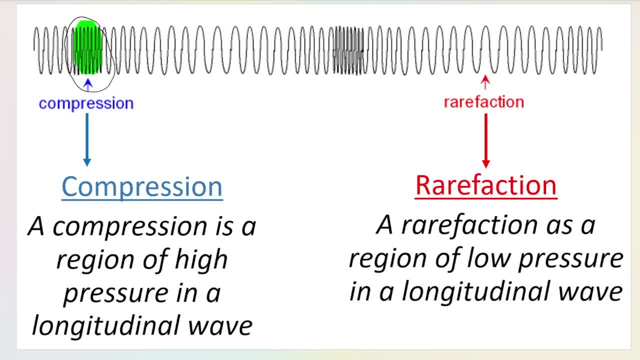 and a rarefaction. So this is a compression. this is a compression. this section over here is what we call a rarefaction, And a rarefaction is a region of low pressure in a longitudinal wave. So think about it: where it's all bunched up tightly like that, that's a compression. 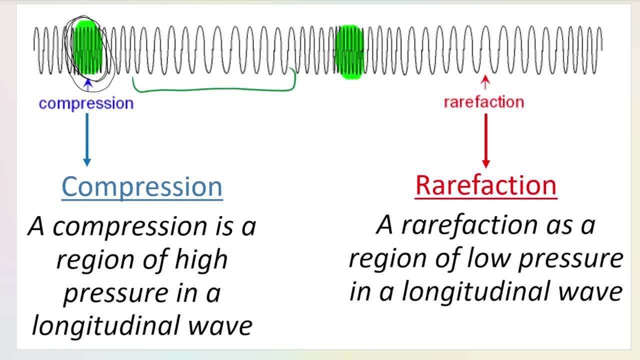 And where it's loose like this. that's a rarefaction. And what do you think this corresponds to if I have to think about a transverse wave? Remember, a transverse wave looks like this: Remember, in a transverse wave we have crests. 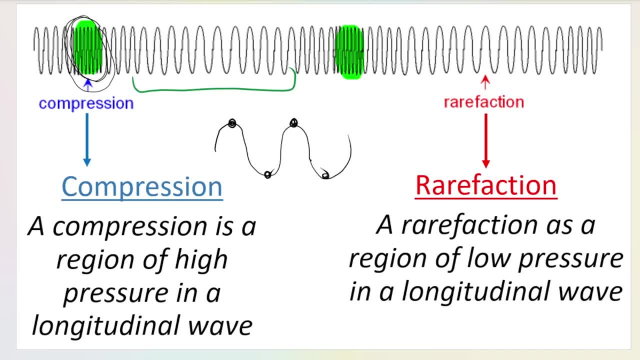 and we also have a wave. So if I have a transverse wave, I have a wave. So if I have a wave, I also have troughs. So what I want you to think of it is like this: the areas of high 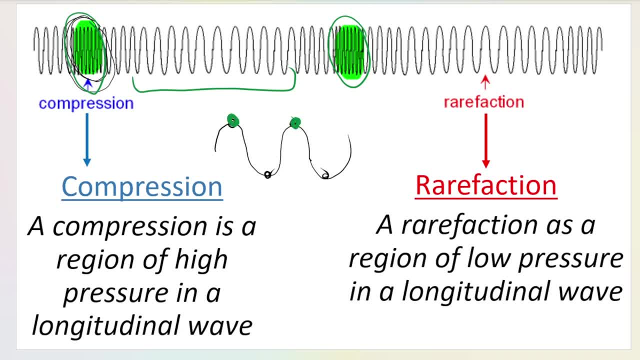 pressure. so the compression, that's like a crest, crest compression, and the regions or the areas of low pressure, the rarefactions, that's like a trough. So what's important to note and remember? when we did transverse waves, we said the distance between two successive points in phase or two. 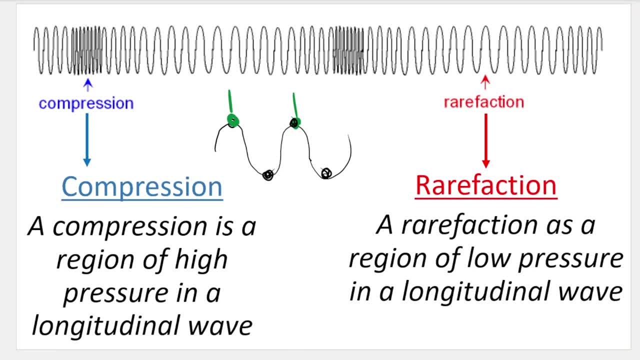 successive crests, In other words one crest that comes after the next. So if I have a transverse wave, the distance between those that gave me what I call the wavelength in a transverse wave And it works similarly in a longitudinal wave. If I take the compression over here, the middle of the. 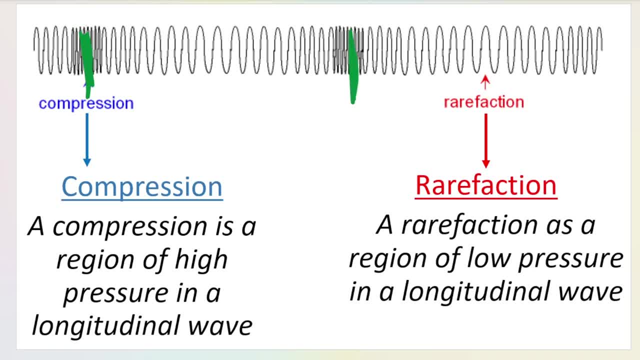 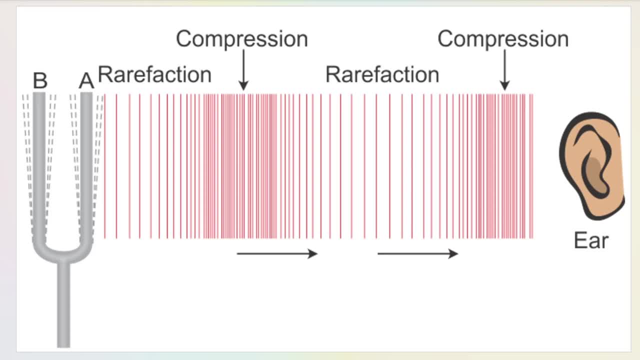 compression over there and the middle of the next compression. those are two points in phase. If I connect those points, that will give me the wavelength of the wave. Okay, so here's another diagram to illustrate compression and rarefaction, And just so you know. 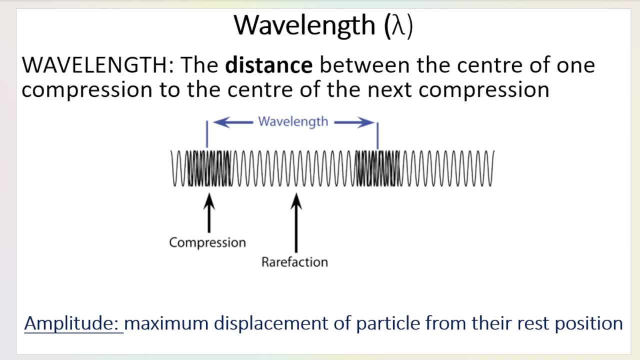 like I showed you the distance between the center of one compression and the center of the next compression, that is the wavelength. So they can ask you to work out the wavelength for a longitudinal wave. It would be the distance between the center of this compression and the center of this. 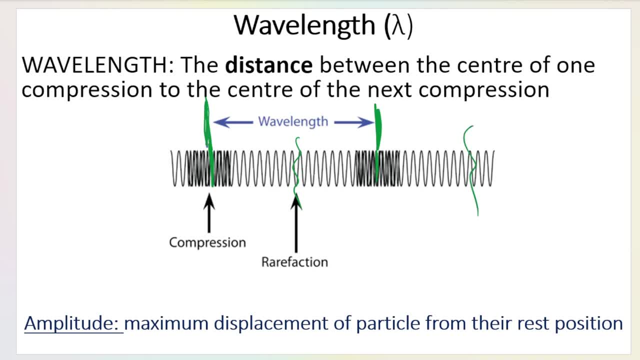 compression, or the center of this rarefaction. and the center of this rarefaction. Now, what is amplitude? Amplitude? just like with transverse waves, amplitude is the maximum displacement of a particle from its range. So, if I take the distance between the center of this compression, 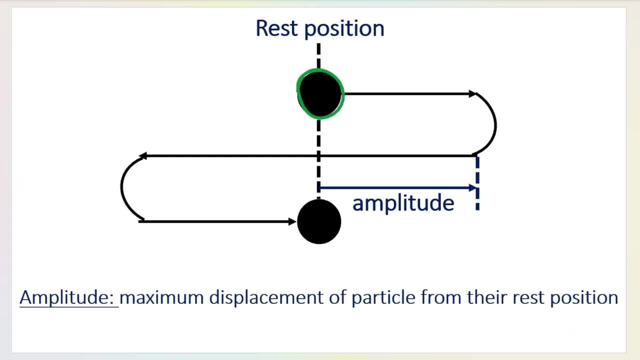 and the center of this rarefaction, that is the maximum displacement of a particle from its range. So remember: here the particle starts out in its rest position, then it's displaced, In other words it moves to its maximum distance away from that rest position. That distance over there is called 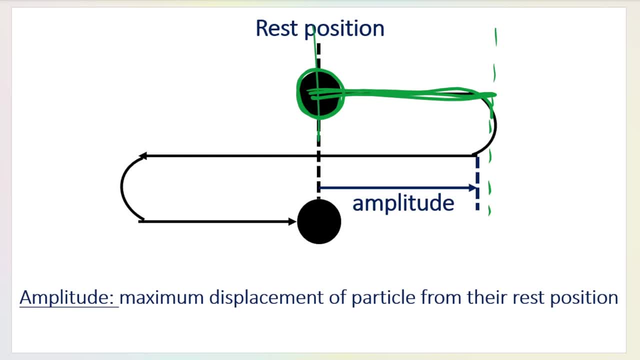 the amplitude. Then it does the same thing in the opposite direction. Here's its rest position, Here's its maximum displacement in the other direction. Again, that distance is called the amplitude. Right Now, what are the properties of the wave or variables relating to the amplitude? 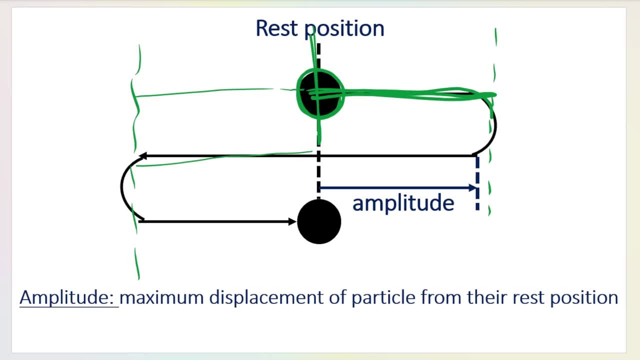 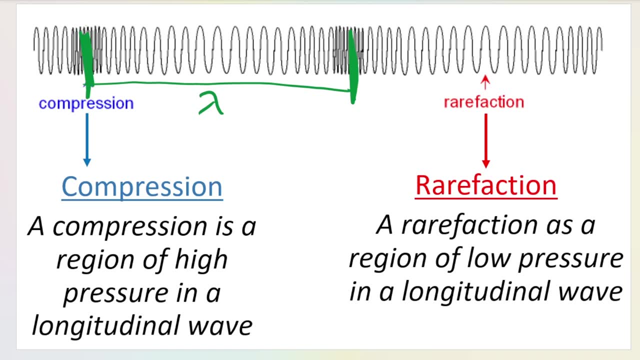 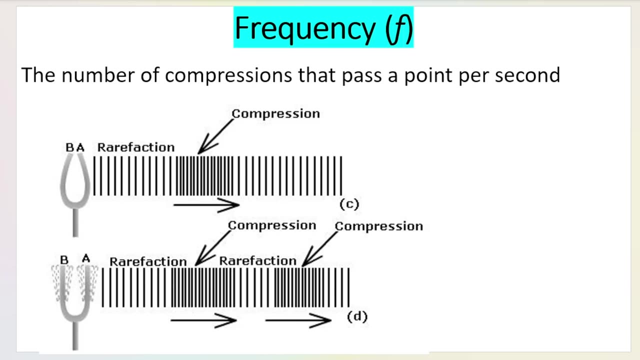 of the wave. can you remember from transverse waves? so we've spoken about amplitude, we've spoken about wavelength, we've spoken about compression and refraction, which corresponds to the crest and the trough. do you remember frequency? well, remember the frequency of a transverse wave. that was the. 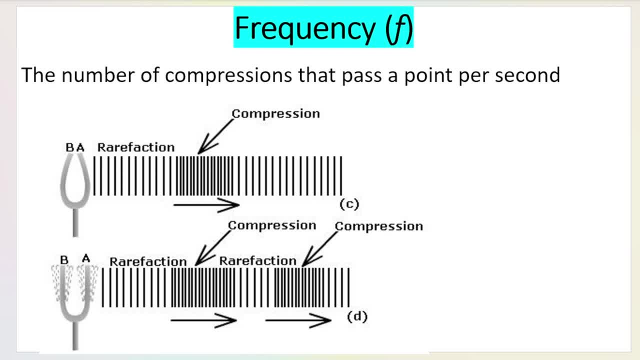 number of wave pulses that pass a point per second, or the number of crests that pass a given point per second, or the amount of wavelengths that pass a point per second. so the frequency of a transverse wave is very similar to the frequency of a longitudinal wave. for the frequency of a 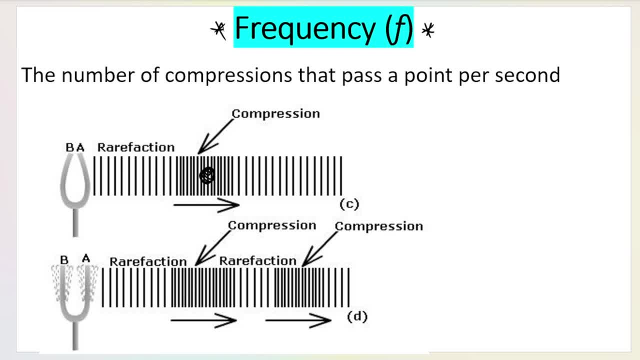 number of compressions that pass a point per second. the number of compressions that pass a point per second. so if i say the frequency is two hertz, it means that two compressions- yeah, one, two- pass a given point in one second. and period was my other variable, or my other quantity and period, remember for a 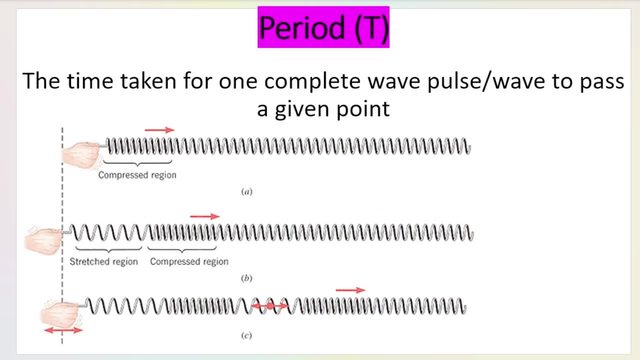 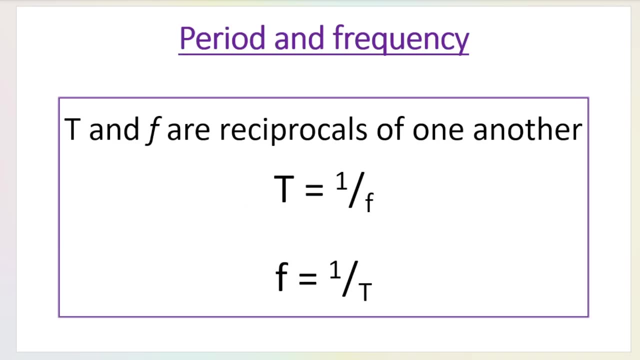 transverse wave was. it was the time taken for one complete wave, pulse or wave to pass a given point. it's the same thing for longitudinal waves. and remember grade 10s. we learned about how period and frequency are related to one another. remember period and frequency are reciprocals of one. 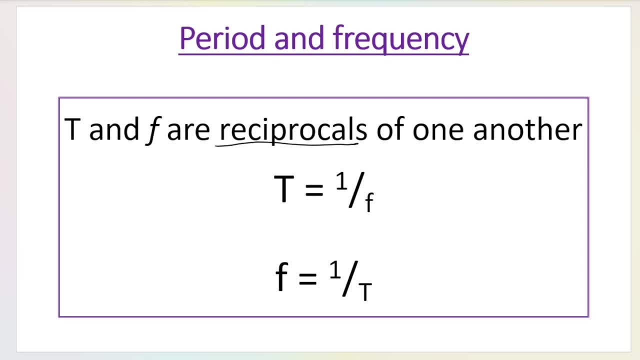 another, which means if i know the frequency i can easily get the period and vice versa. so for example, if i say the frequency is two hertz, then i know the period is one over two hertz. if i say that the period is five seconds, then the frequency is one over five hertz. sorry, this period that. 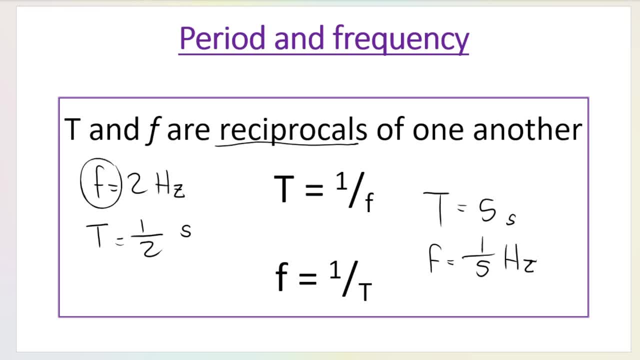 unit over, there should be seconds. okay, so the unit for frequency is hertz and my unit for period is seconds. there are reciprocals. so if i tell you the frequency is two over three hertz, you can tell me: oh, the period is three over two seconds. reciprocal means i flip the fraction, but we 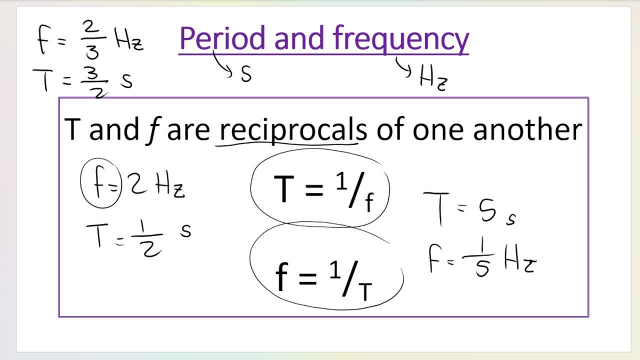 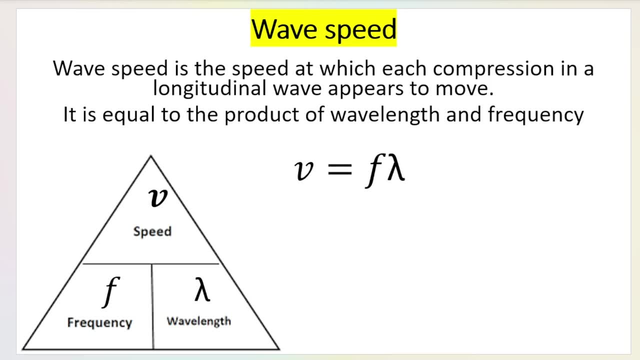 also have these formulas that i can use to calculate it. and, just like we did with transverse waves, we can work out the wave speed for a longitudinal wave. all we need is the frequency and the wavelength. so it says. the other wave speed is the speed at which each compression